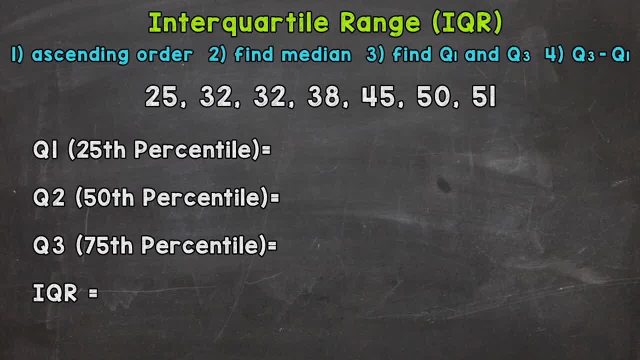 median. Now steps two and three are going to be the same, but we're going to do a data set with the median and the median. So we've got an odd number of numbers and we're going to do the median in ascending order, which means least to greatest. So the first thing we want to do is 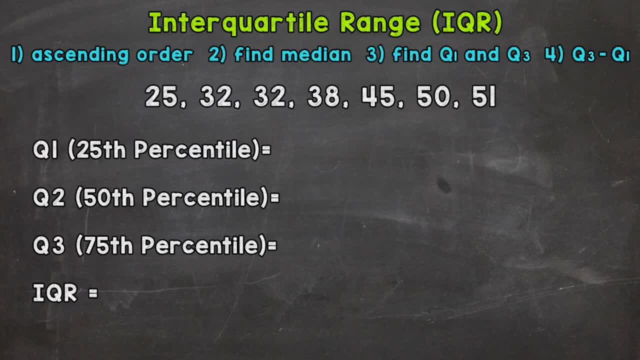 find the median. Now we want to see if we can find the median in ascending order, and that is to find the median as far as finding quartiles. So the median is the middle of our data set. In the case of this example, we have seven numbers, so we will have three numbers on the left, three. 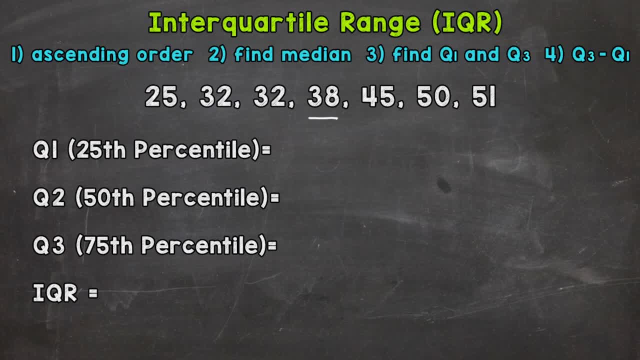 It's going to be 38.. So down here, where it says Q2, 50th percentile, I'm going to write 38. Q2 stands for quartile 2, which is the same as the median. So Q2: 50th. 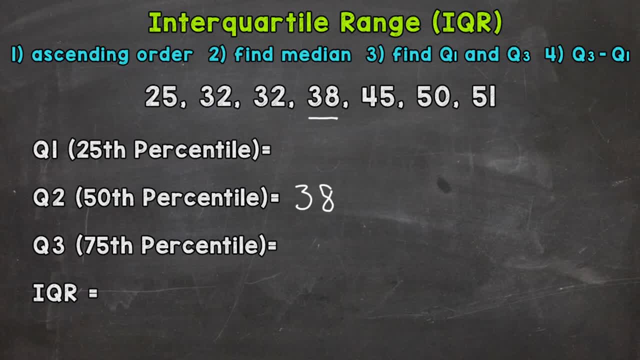 percentile and median all mean the same thing. So once we have the median, we can find the lower and upper quartiles. Let's start with the lower, So we'll take a look at the lower half here and we need to find the middle of that lower half. 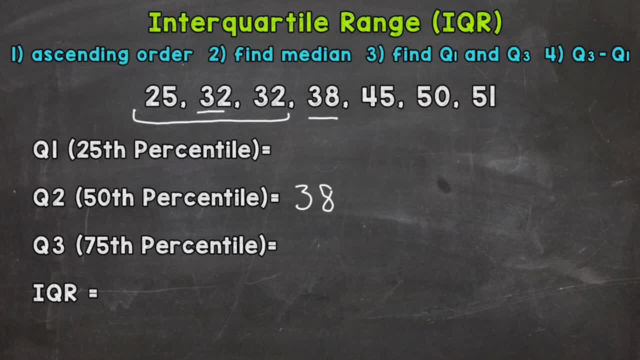 the median of the lower half. It's going to be this 32 here. Since we have three numbers, it's going to be the middle one, So Q one quartile. one means lower quartile, So let's write 32.. Upper quartile: we will take a look at the. 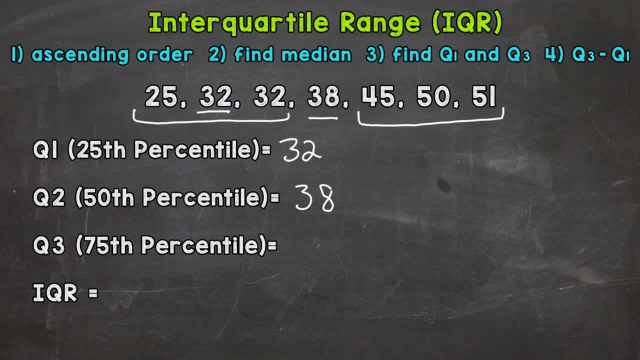 upper half and find the middle or median of that upper half and that's going to be our upper quartile. So it's going to be that 50. So our upper quartile is 50. Once we have all of that information, we can find the interquartile range. 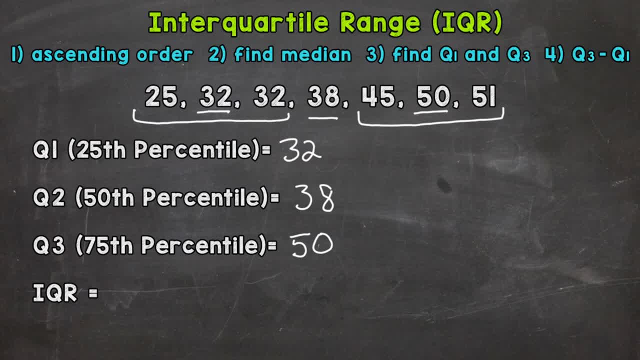 We take our upper quartile and subtract the lower quartile, So our upper is 50 minus our lower, which is 32.. So 50 minus 32 gives us an interquartile range of 18.. So I'm going to draw some lines within our data to help us visualize exactly what this all means. 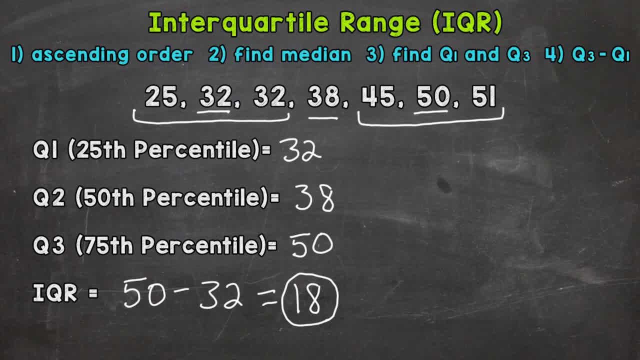 So our median was 38. So let's draw a line there. Now, remember, when we find quartiles, we're splitting our data into quarters or four equal parts, And our interquartile range is the range of that middle 50%. So our lower quartile is 32.. Let's draw a line there. 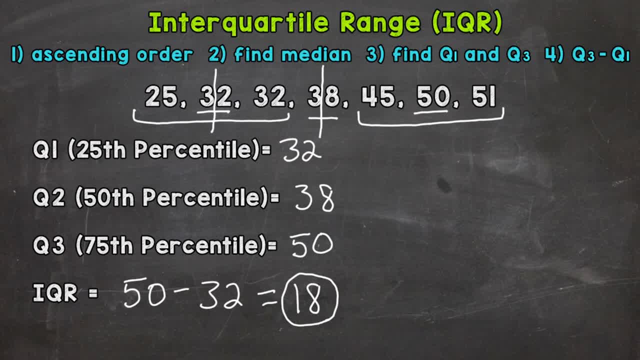 And then our upper quartile is 50. So you can see that we have our quarters, or four equal parts there. What we do when we take a look at the interquartile range is: look at this section here, Our middle 50%. 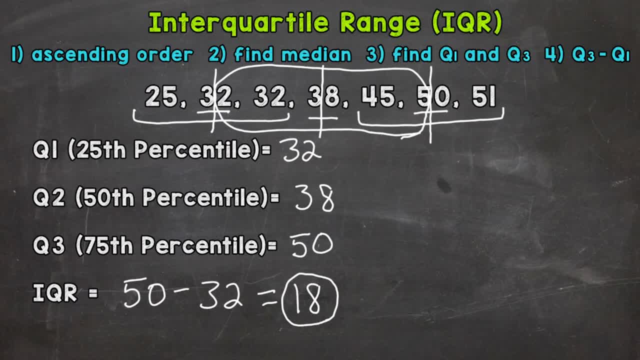 So we found the range or difference between 50 and 32.. Our upper quartile and lower quartile. So that gave us that interquartile range. Let's move on to number two and do another example. So for our second example, we're going to have a data set with 10 numbers. 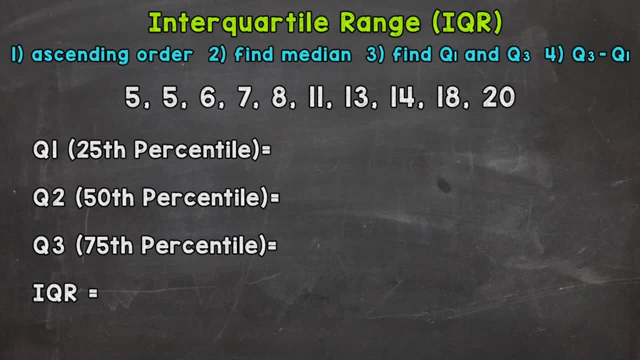 So remember, the first thing we want to do is put the data in order from least to most. This data is in order as well, just like the first one, So we can move to the second step, which is find the median. Now that means the middle. 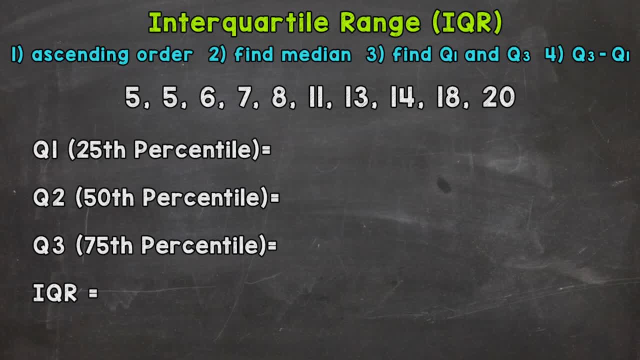 In the case of this number, we have 10 numbers in our data set, So we're going to break it in half, the midpoint. So we have five numbers on the left and five numbers on the right. So our median is going to be right here between 8 and 11.. 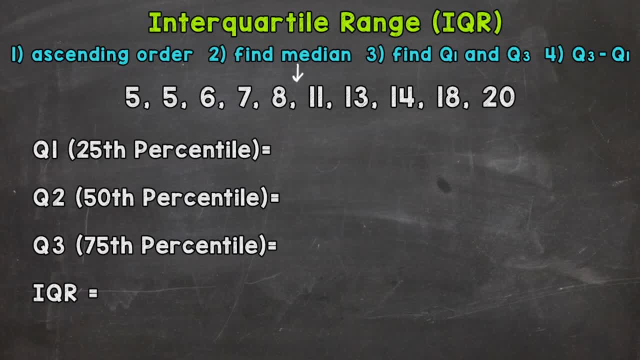 It's between two numbers there. So how we find the middle? we need to find the average of 8 and 11, and that's going to be our median. So we can do that by adding 8 plus 11 and then divide by 2.. 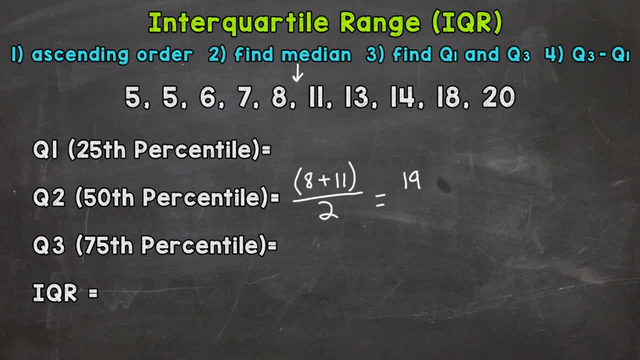 So 8 plus 11 is 19, and 19 divided by 2 is 9 and 5 tenths or 9 and a half. So that's our median. Let's do our lower quartile next. So we need to take a look at the bottom half here, the bottom five numbers, and find the middle or median.